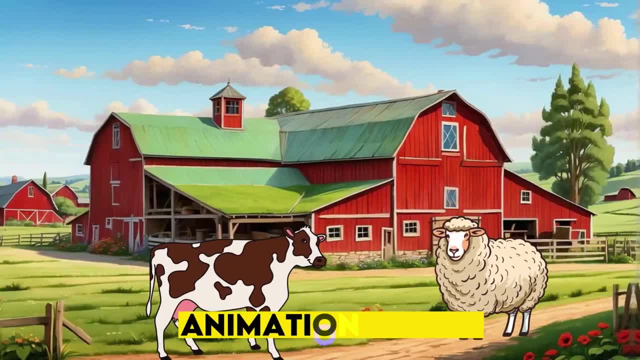 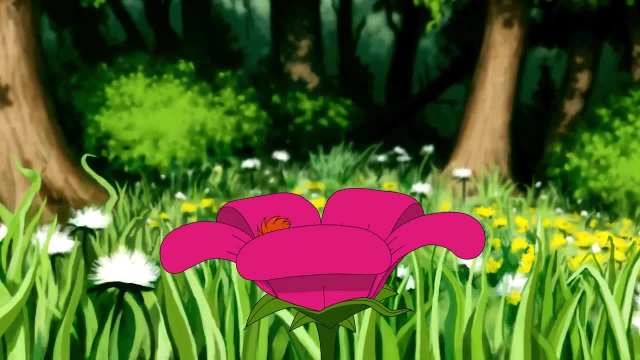 In today's video, we will learn how to create kids' learning animation videos, starting from the script, image generation, voiceover and the final animation video. We will walk through each and everything in detail, So, without further delay, let's get started. 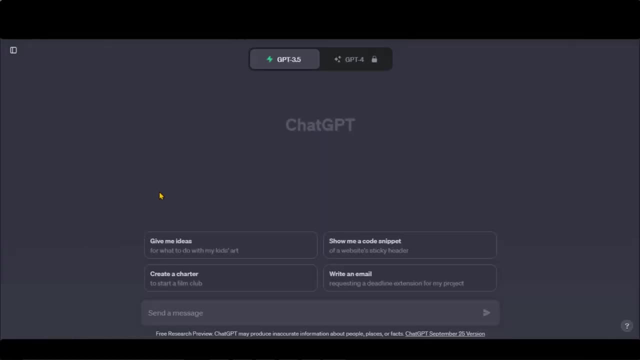 First, we will generate a script by using ChatGPT and BARD AI. Go to ChatGPT and type this simple prompt. Here I have typed the title of a story, the characters we will use in this story and, of course, the background scenes. 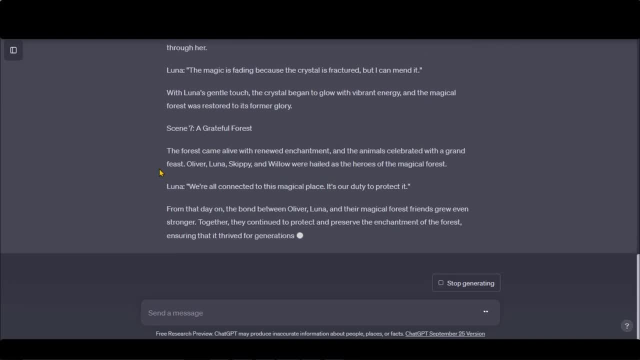 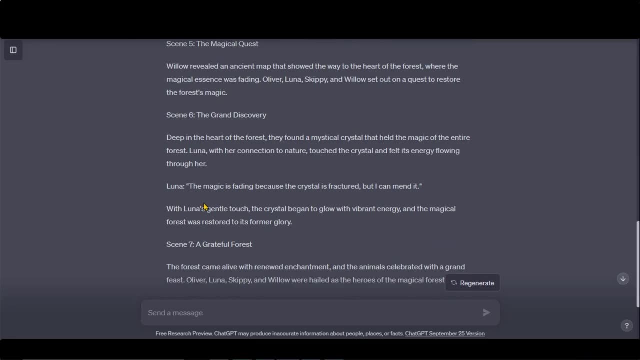 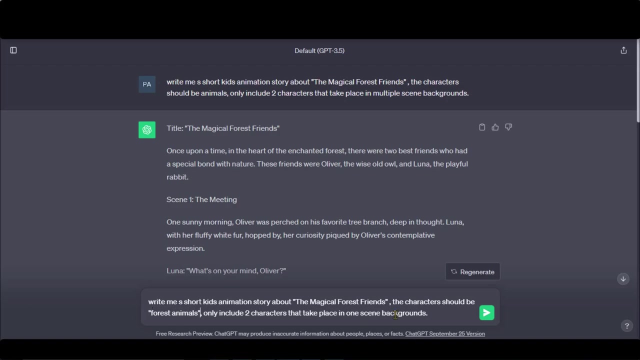 Press the Enter button and wait for the process to complete. Here we have our script. It looks good to proceed. Let's change the prompt by specifying the animals and only a single scene background. This script also looks fine. You can write it in a better way. 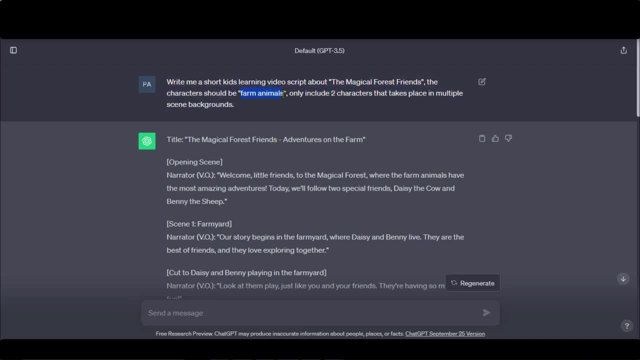 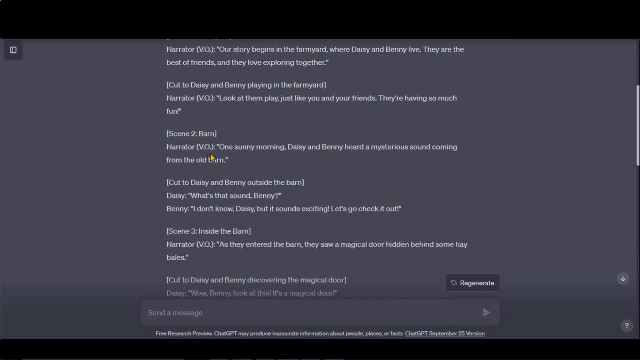 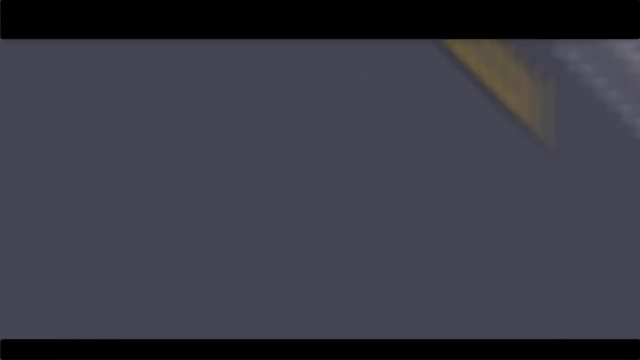 Here I have changed my characters to farm animals. You can see the final script with complete scenes and dialogues between the characters. That looks perfect to proceed, So you can improve the script by applying different commands. Copy the same prompt and go to BARD AI. 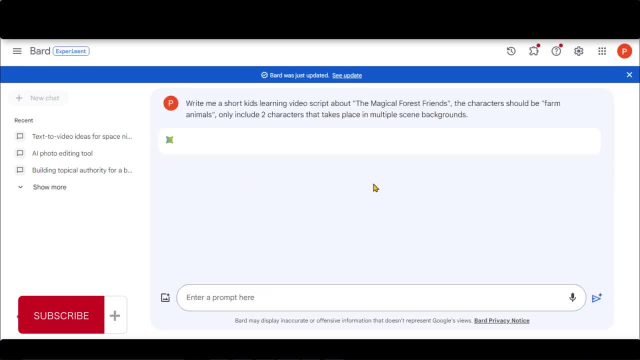 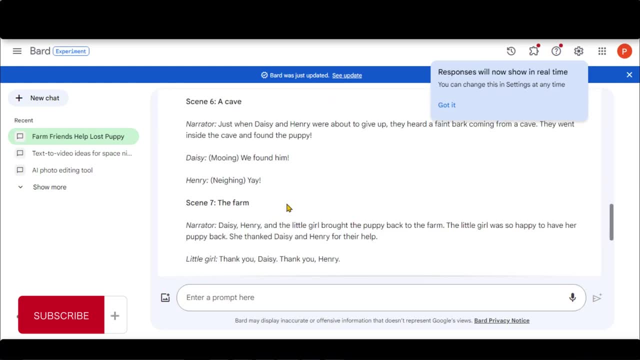 Paste your prompt here and click on the Submit button. Press the Enter button and you are good to go. Look at the final result. You can compare both the prompts, So you can proceed according to your choice. Let's move to the next part: generating voice over and sound effects. 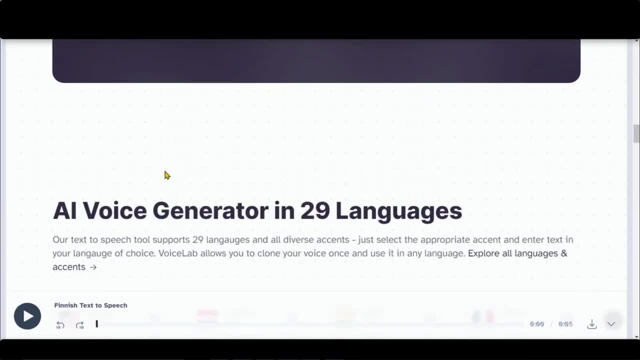 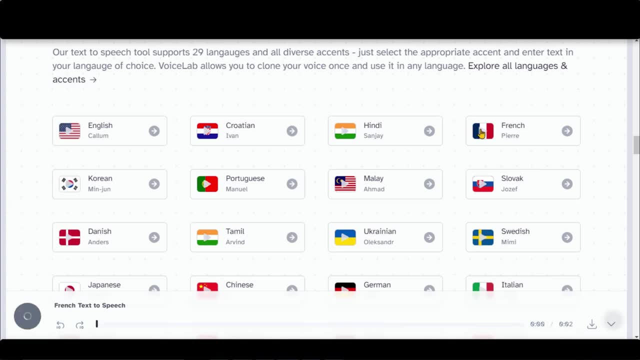 We will use 11 labs for voiceover. It can generate voices in 29 different languages. Sometimes it is better to lose and do. You're beautiful when you don't want to beat your code To tell these words. you often get too lazy. 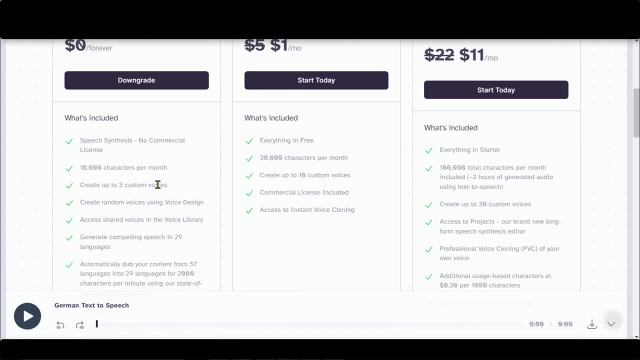 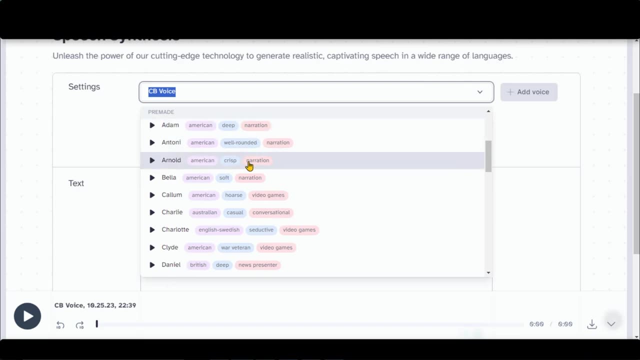 With a free plan, you have 10,000 characters per month with with limited features. Its Starter Plan gives you 30,000 characters and some exciting features, such as commercial access and voice cloning. You also have access to the pre-made voices for different categories. 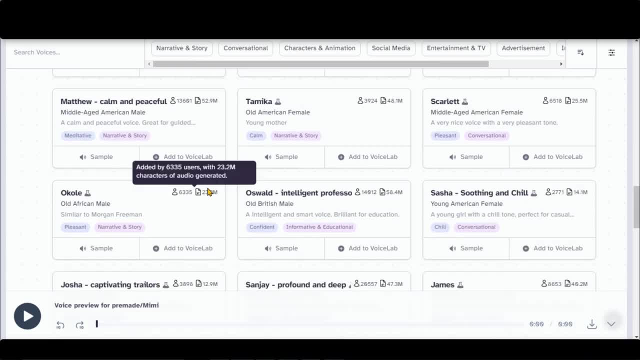 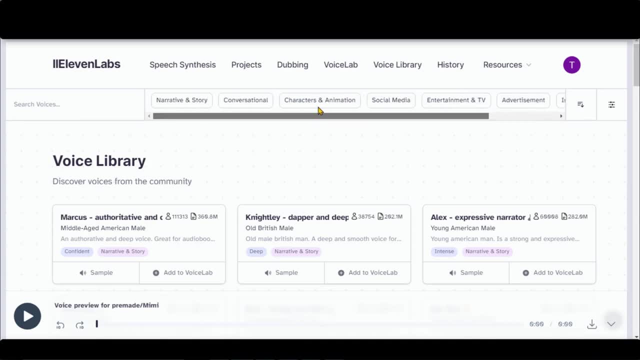 In the Voice Lab you have access to a variety of voices. You can filter them by different categories. This feature is only available in the Starter Plan. Let's select Character and Animation. Here you can listen to the voices. Everyone thinks of changing the world. 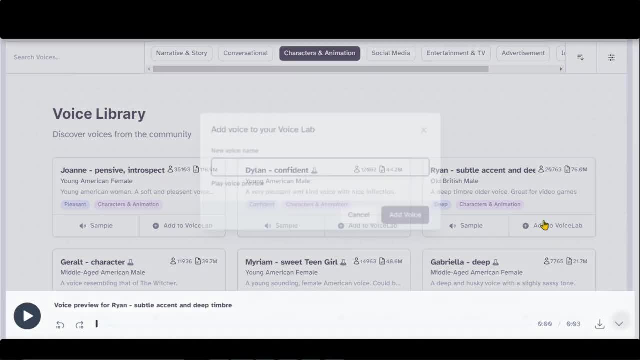 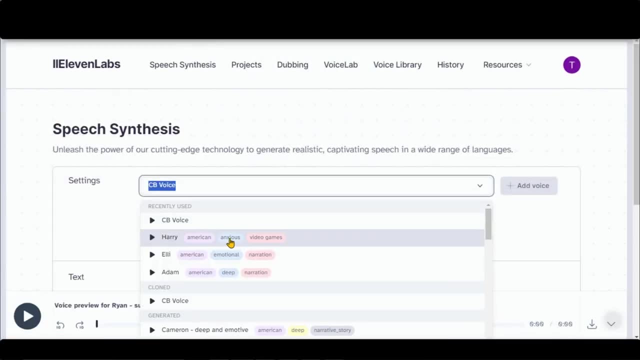 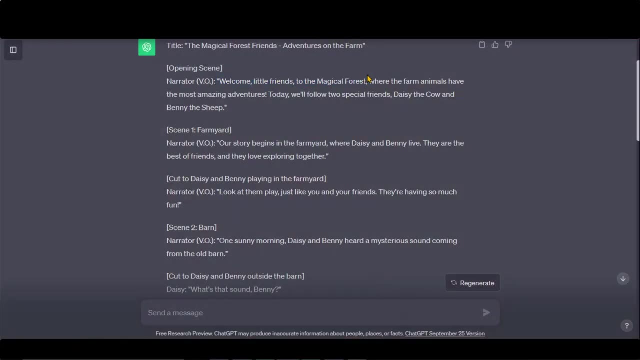 As an organizer, I start from where the world is. Click on this plus icon to save it to your library. On the main dashboard, you can access your saved voices. Select your voice. Also, you can adjust the settings. Copy the scene's narration one by one: 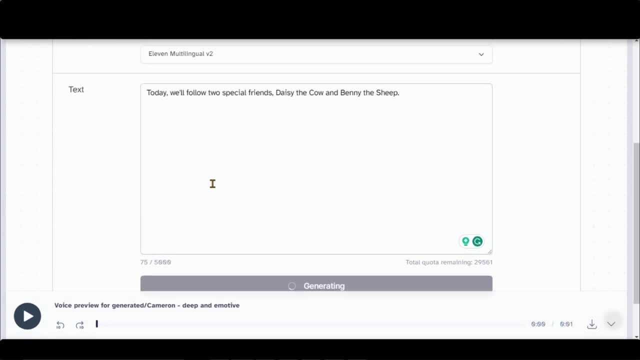 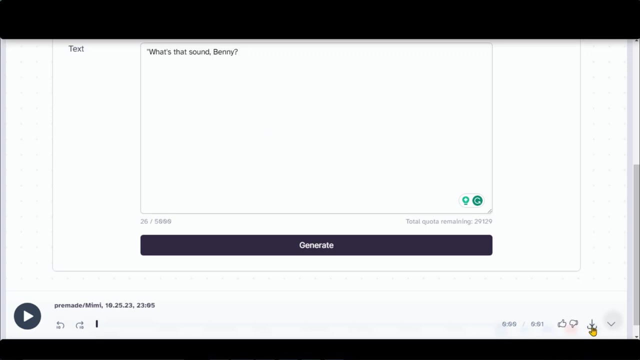 and generate the voice. Today, we'll follow two special friends: Daisy the Cow and Benny the Sheep. Now change the voice artist for the cow and sheep, Generate the voice and download it. What's that sound? Benny, You can repeat this process for the whole script. 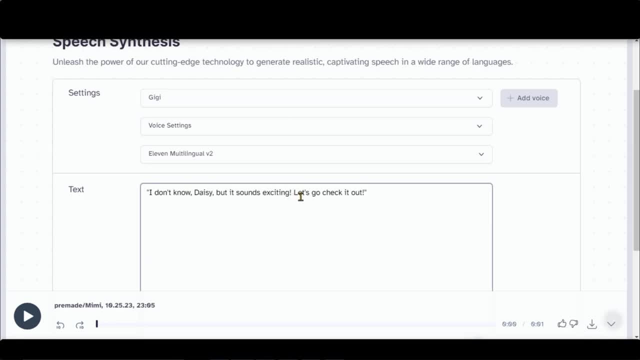 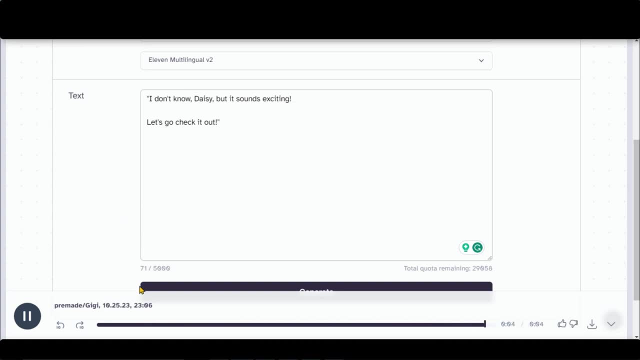 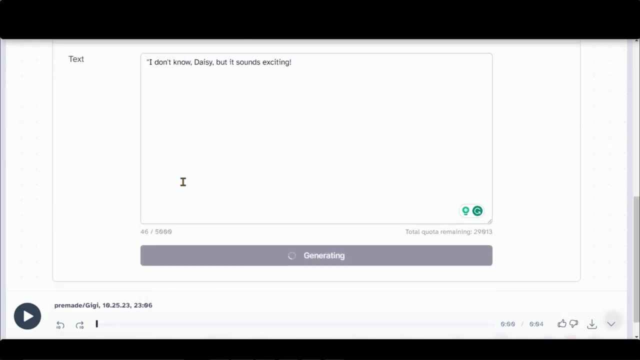 Sometimes you do not get the desired result for a voice. I don't know, Daisy, But it sounds exciting. Let's go check it out. Just adjust the settings a little bit and you will be able to get the perfect voice. I don't know, Daisy. 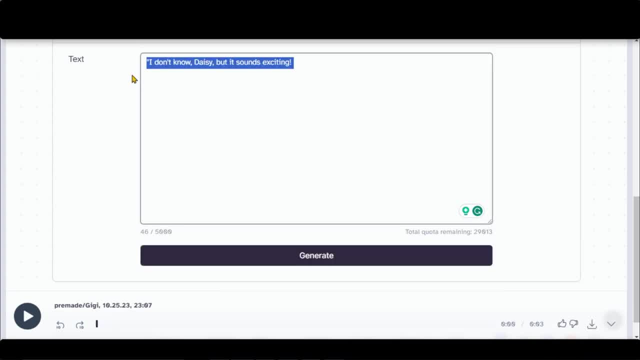 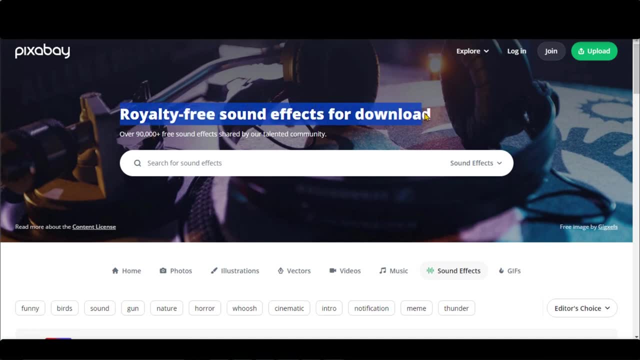 But it sounds exciting, So you can play around to generate a complete story-based voiceover. Pixabay is an amazing and free platform for sound effects. Almost 90,000 plus royalty-free sound effects for all types. Let's find a cow voice. 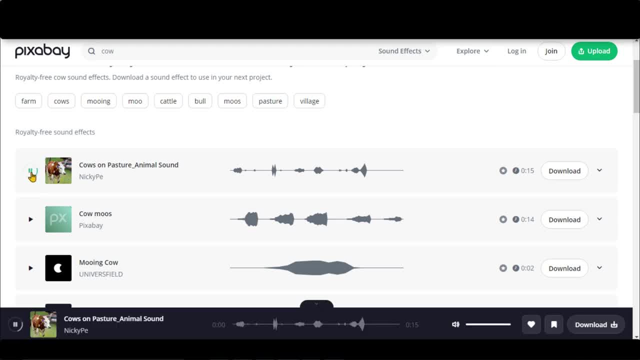 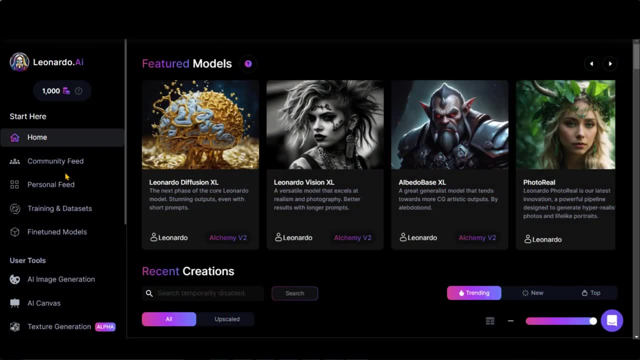 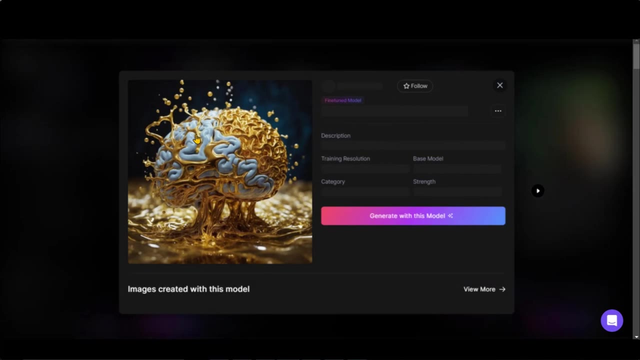 Here you can see the results. Click on it and listen to the voice. Click on the download button to save it to your computer. For image generation, you can use Leonardo AI and DAL E3.. We will cover both in this video. Leonardo AI has introduced some new models and features. 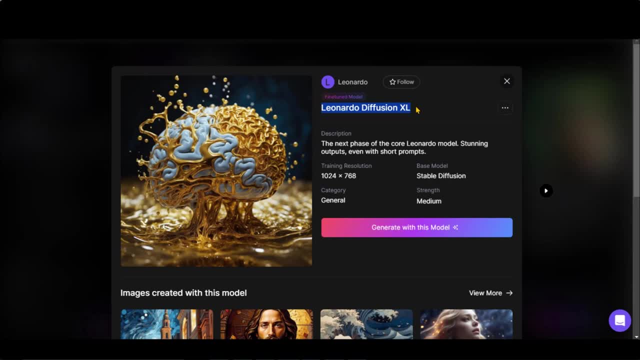 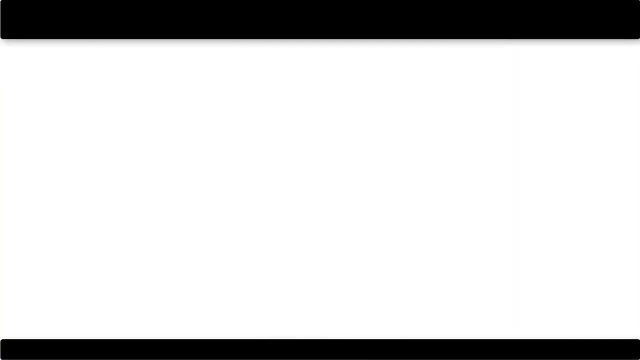 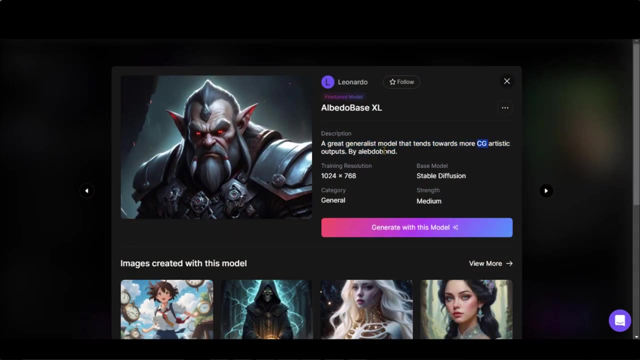 Right now they have added these three models based on stable diffusion. The first model also works best with short types of prompts. Here you can see some of the results. This model is for realism and photography type of images. The last model gives you some CG artistic output. 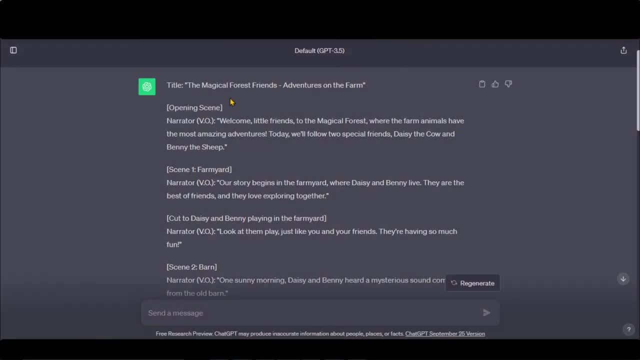 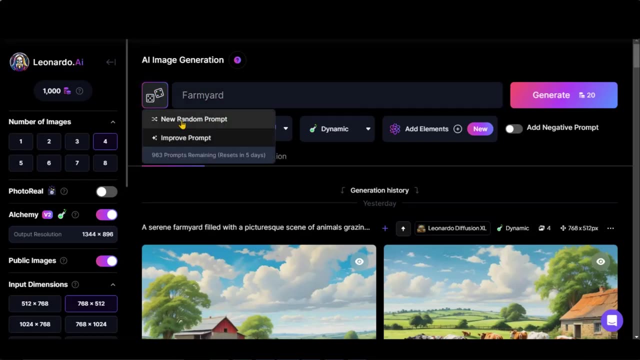 You can analyze the results here. Let's generate the images based on the script. Copy the text, Click here and you will see these two options: to generate a random prompt or improve the existing one. Let's choose the first one. It has completely changed the subject. 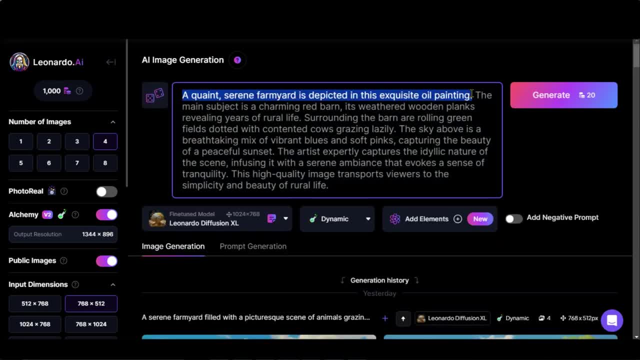 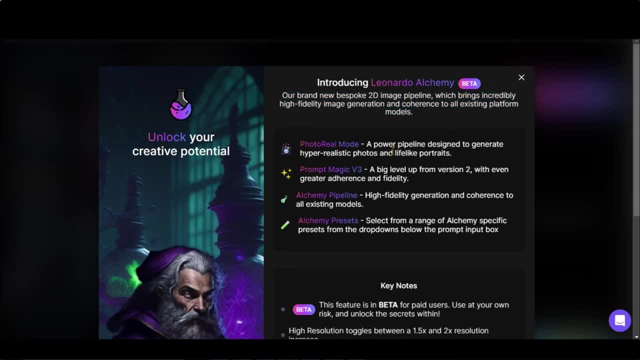 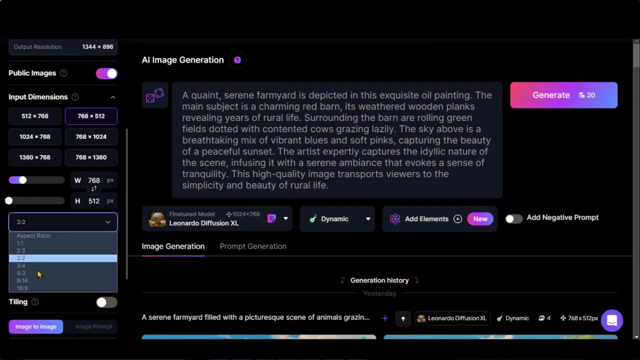 Let's choose the second option. Here we have a detailed prompt: Choose the number of images. Leonardo has improved its alchemy and added some new features available only for paid users right now. Change the aspect ratio to landscape mode. Choose this fine-tuned model. 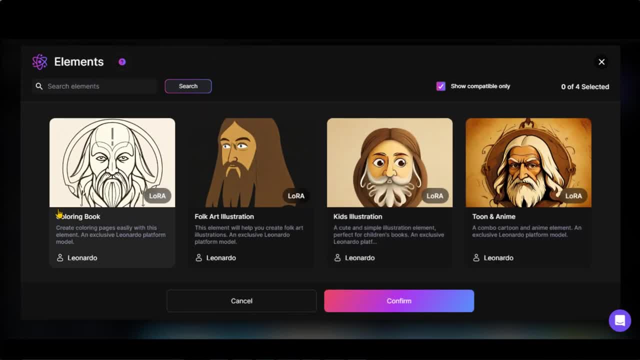 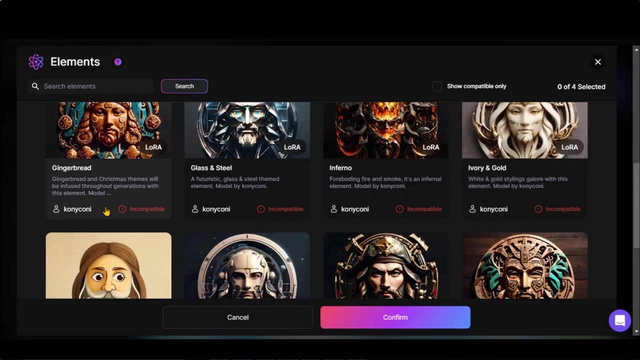 Another new feature by Leonardo AI is Elements to create the specified type of images, such as illustrations, coloring pages, kids illustrations and much more. Currently, these four are compatible with our plan. Here you can see all the available elements. Let's choose this model. 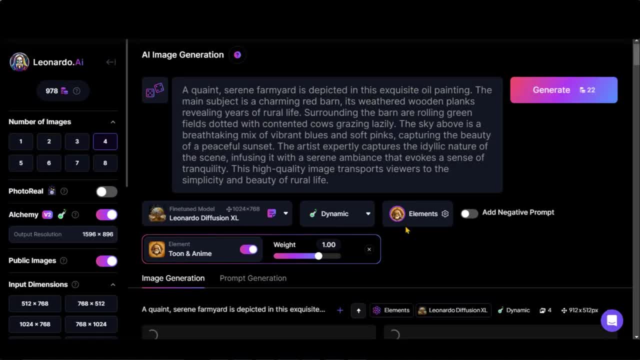 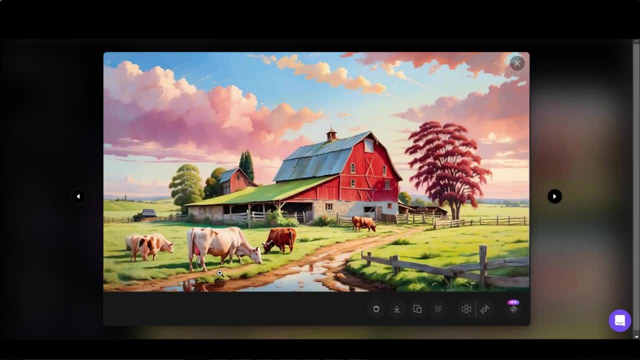 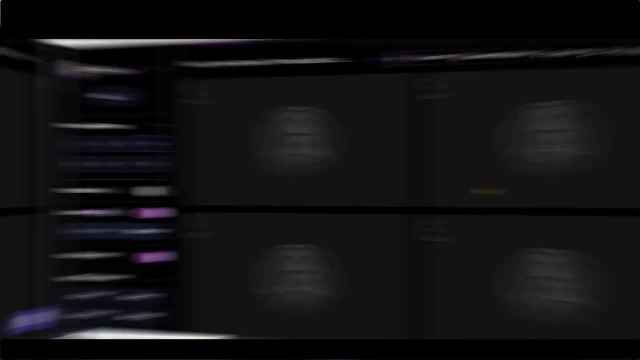 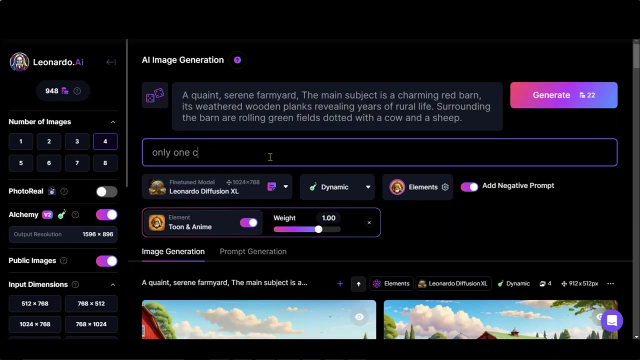 Click on the Generate button. Here you can see the results. Irrespective of animals, these images are amazing. Let's improve this prompt Now. click on the Generate button. Here you can see the final output. Let's activate a negative prompt. 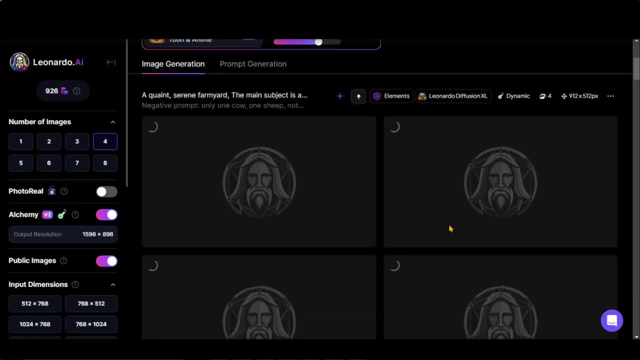 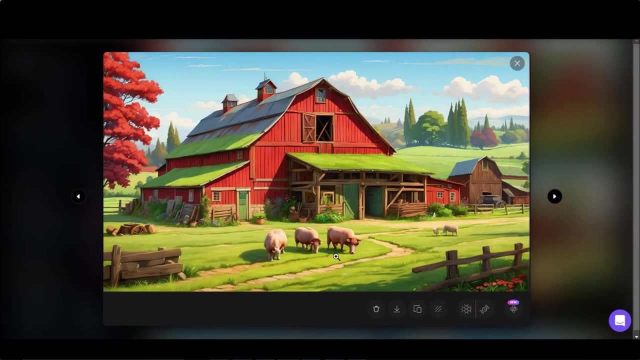 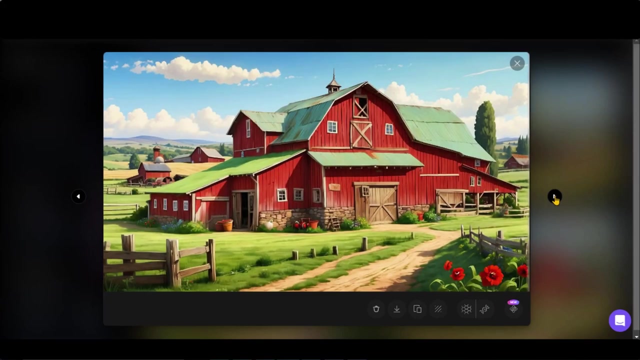 Click on the Generate button and let's see what we get. Here you can see the result. Still, we are getting the animals in the final images. Let's change this prompt a little bit, And here we have the output that we were looking for. 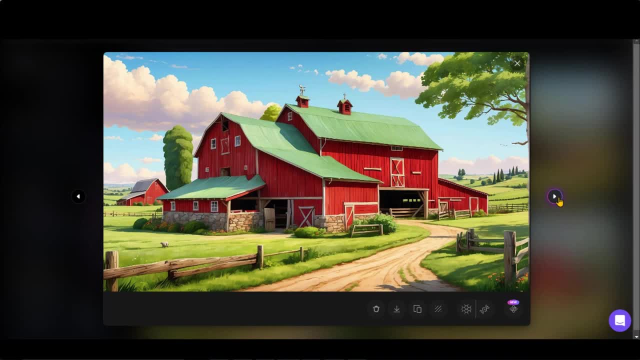 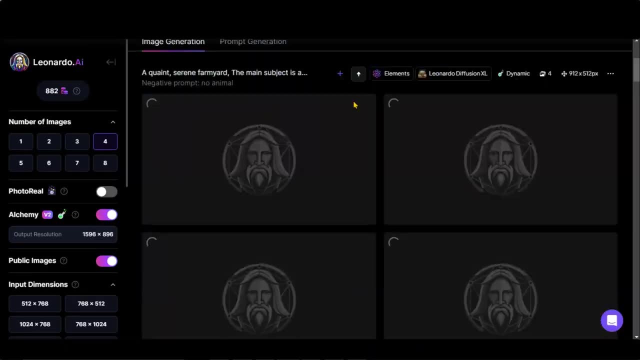 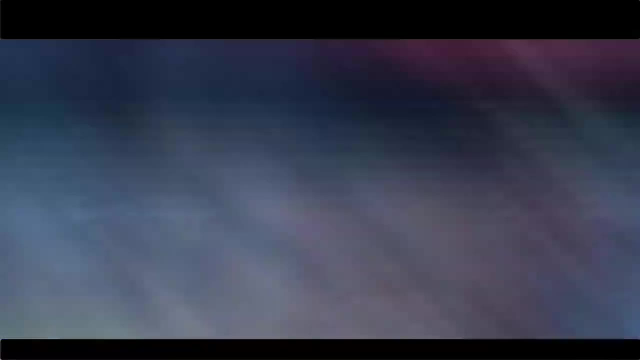 So you can adjust your prompts again and again to get the desired result. Let's copy this text one by one and generate all the images for background scenes. Here we have all the images that we will use in the video. DALL-E3 is another amazing and new AI tool. 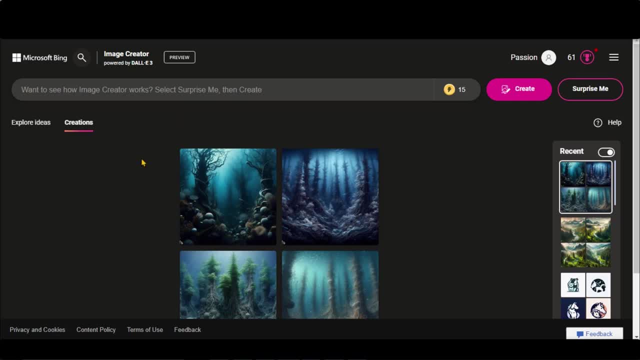 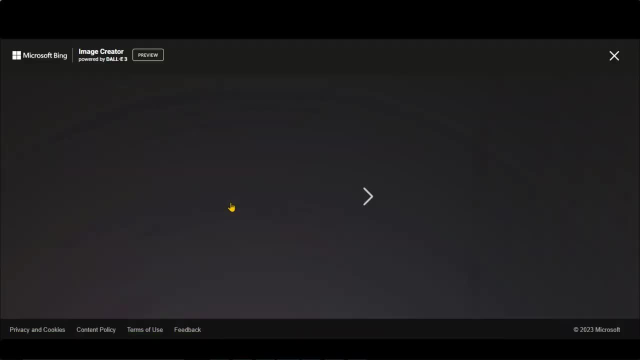 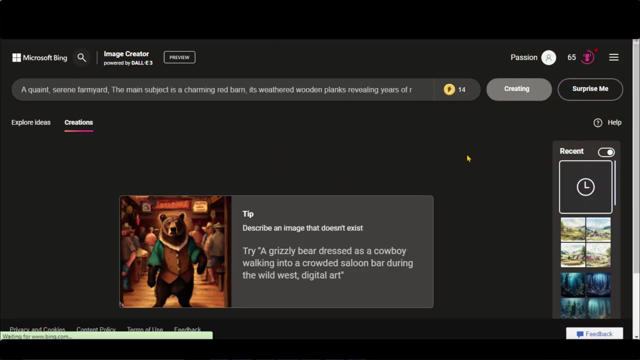 for image generation. You can watch my complete tutorial about this tool by clicking here. Paste your prompt here. Click on the Create button. Here we have the results. Let's paste the detailed prompt from Leonardo AI and let's see what we get. 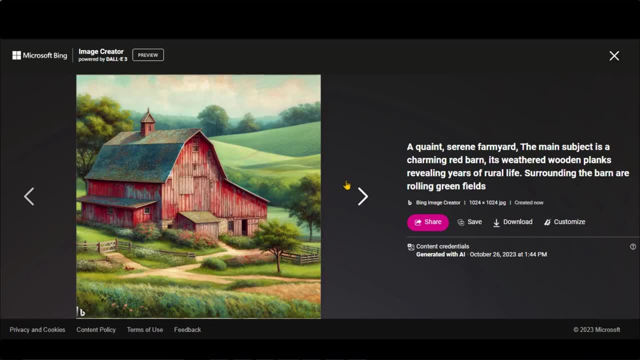 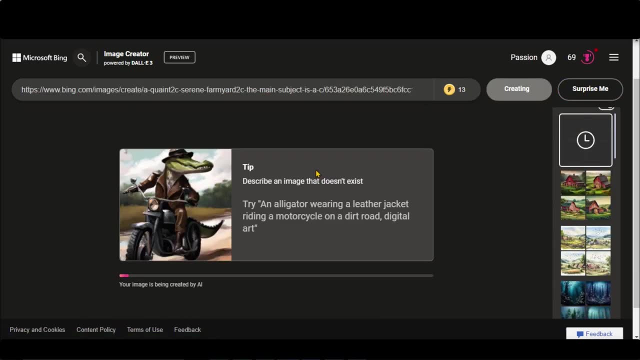 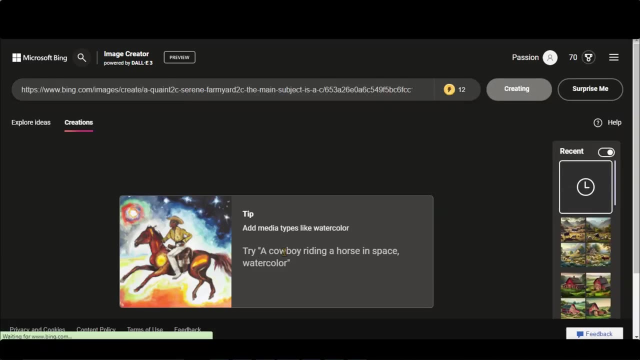 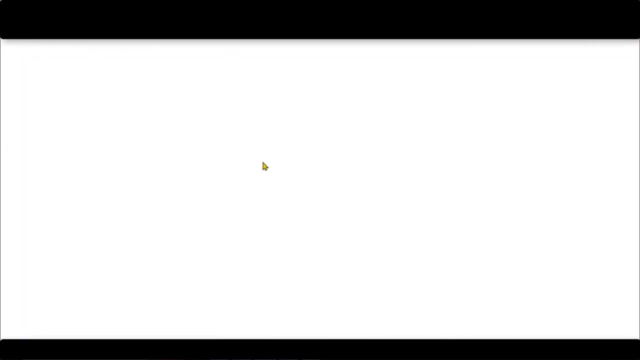 These images are just amazing, to proceed with them. You can drag an image as a reference here and type your prompt to check the results. Make sure to add a detailed prompt to get accurate results. For kids animation, we will use Canva. Go to Canva and choose this video option. 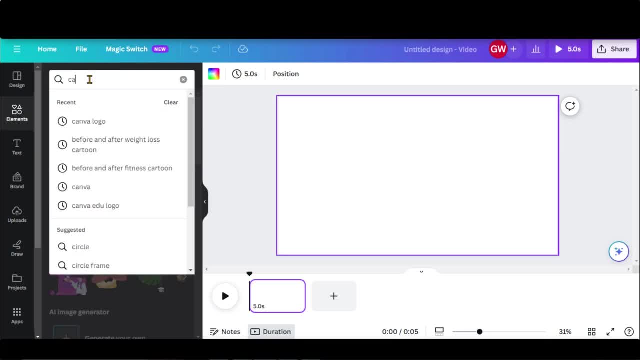 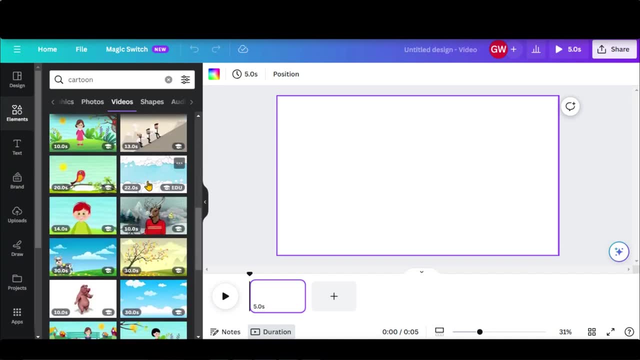 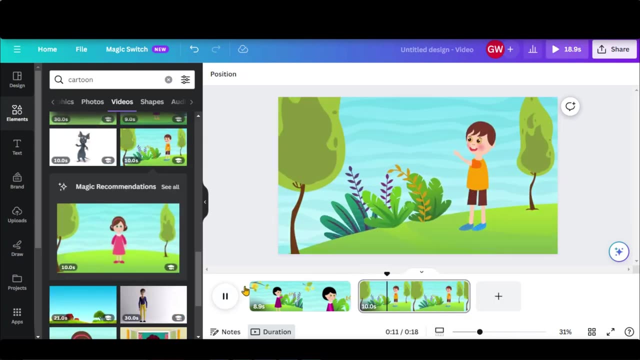 Go to Elements. Type Cartoon in the search bar. Go to the Video tab. Here you have a bundle of pre-made animations. Just choose them according to your script to generate a complete video. Within a few minutes you will be able to generate amazing kids animations. 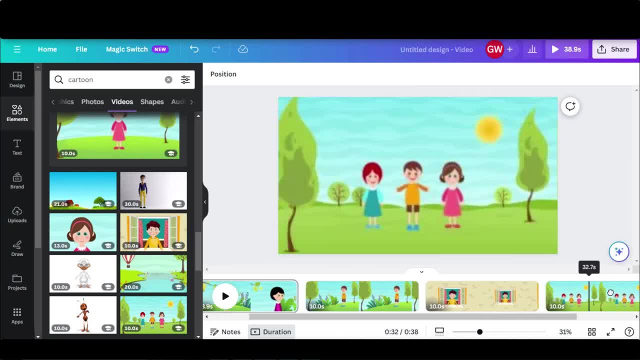 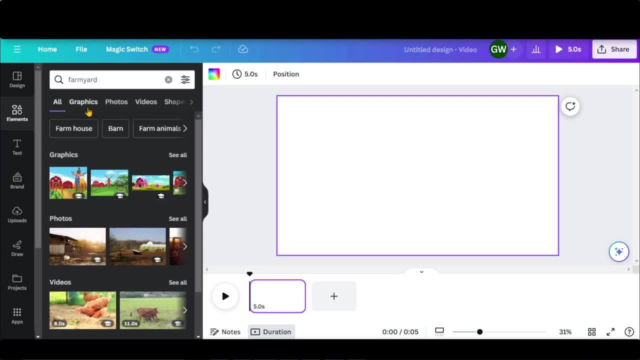 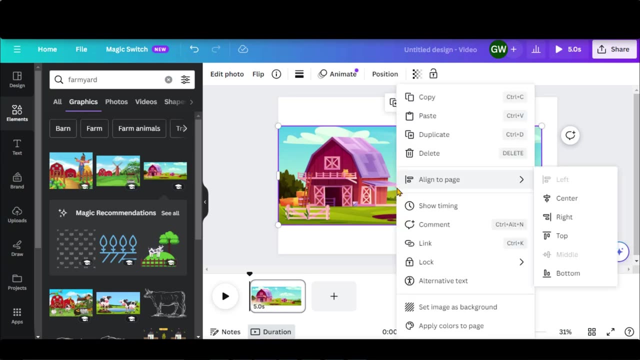 This method is simple and straightforward. Let's move to the detailed and step-by-step process. Go to the Elements and search for the background image for the farmyard. Go to the Graphics and choose any of the images. Resize this image by right-clicking on it. 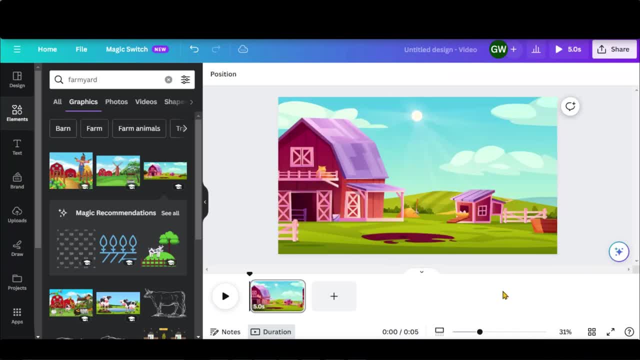 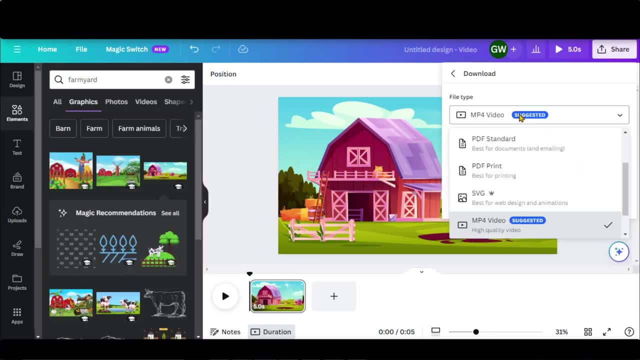 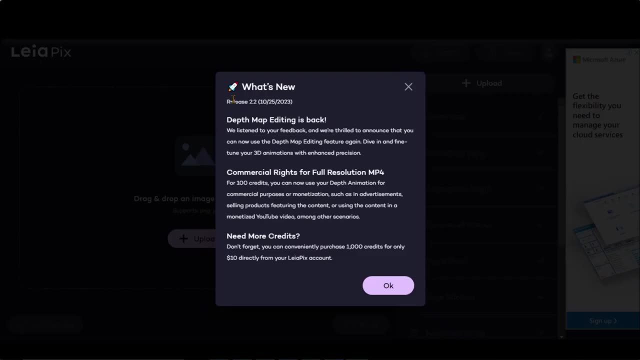 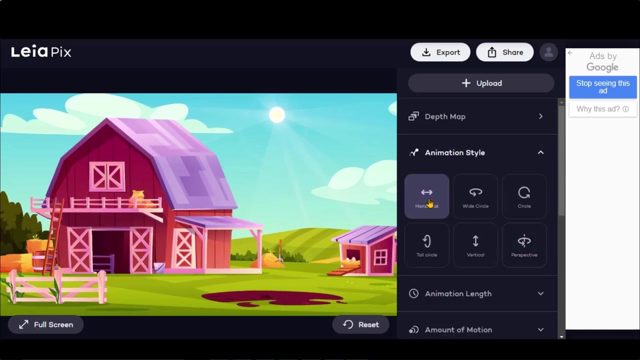 and choose Set as Background. Double-click on it and adjust the image. Download this image as a PNG or JPG to give it an animation background. Leopix is a great tool for animating the images. Just drag your image here. Adjust the animation style. 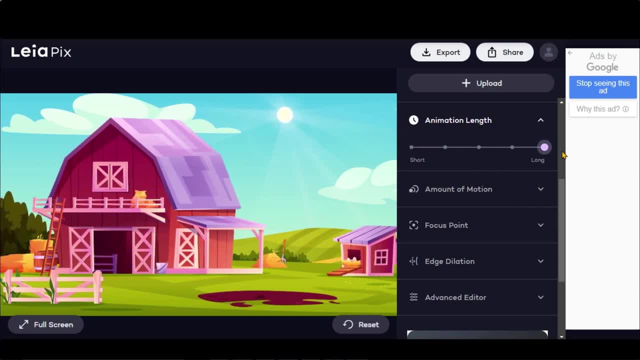 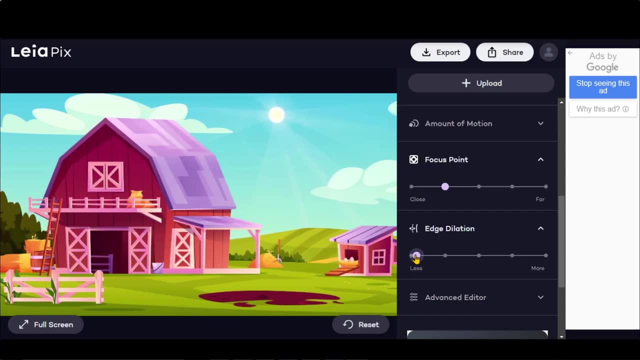 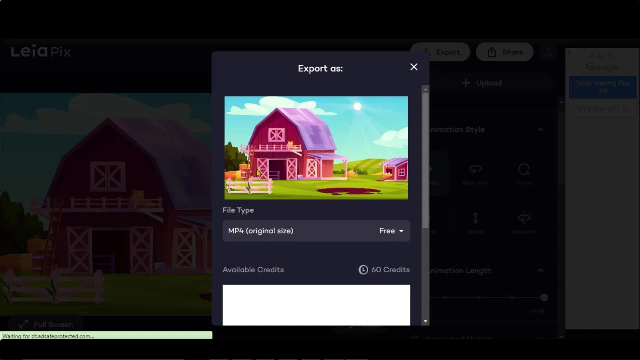 Increase the animation length up to 5 seconds. Decrease the amount of motion, Change the focus point and edge dilation. Here you can see some of the advanced filters. Once done, click on this Export button. You can download the animation up to 720p for free. 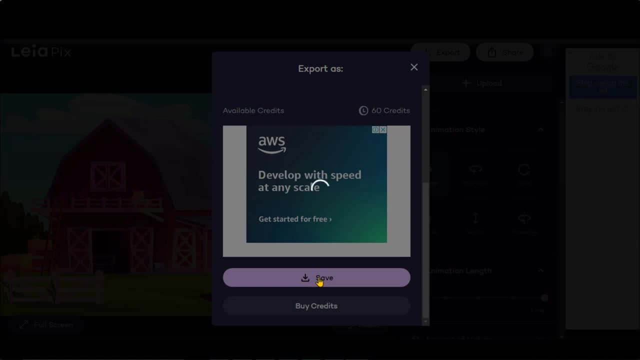 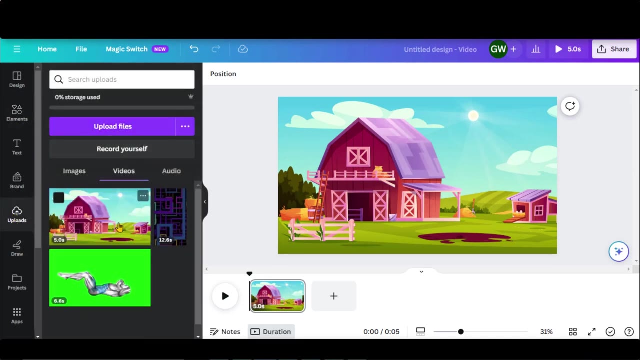 Click on the Save button to download it. You can repeat this process for all the images. Go back to Canva and upload the downloaded file. Right-click on it and set it as a background. Now delete the image. Here you can see a little bit of animated background. 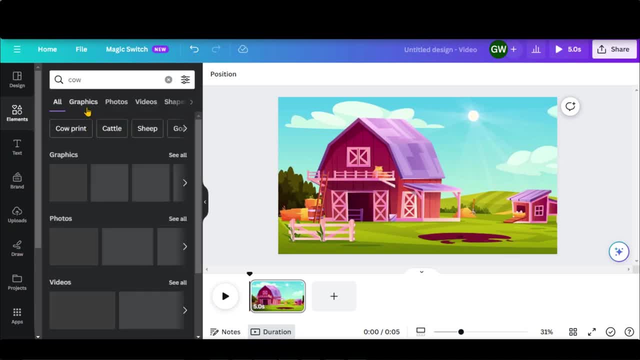 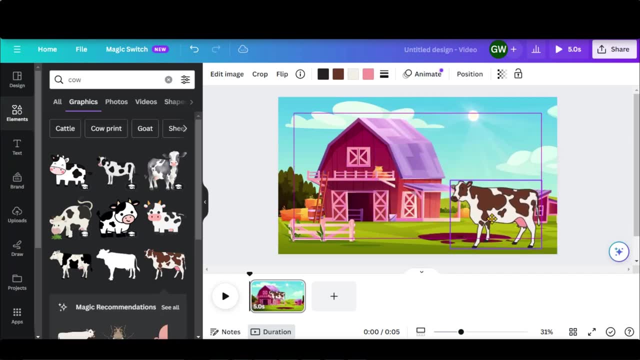 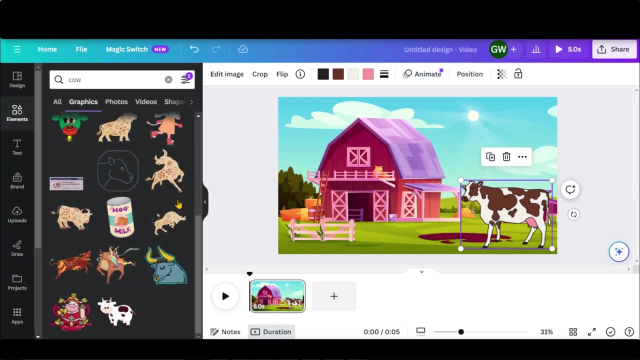 Go to the Elements tab and search for the cow image. under the Graphics tab, Choose any of the images that suit your script. Now adjust it. Click on here and choose Animated. Now you will be able to get some animated images. Now search for the sheep image. 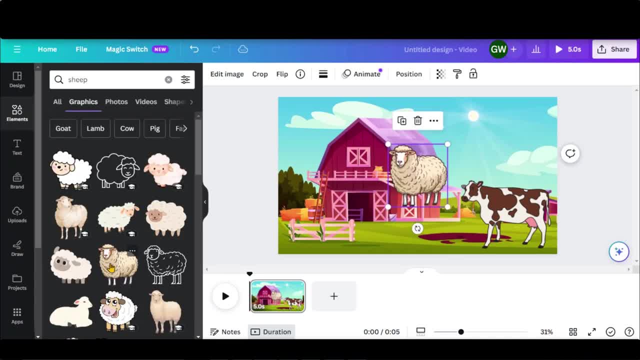 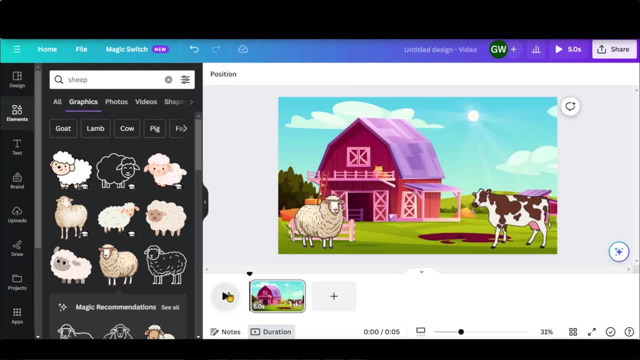 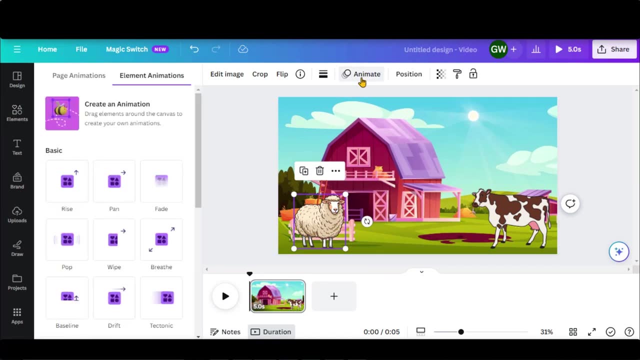 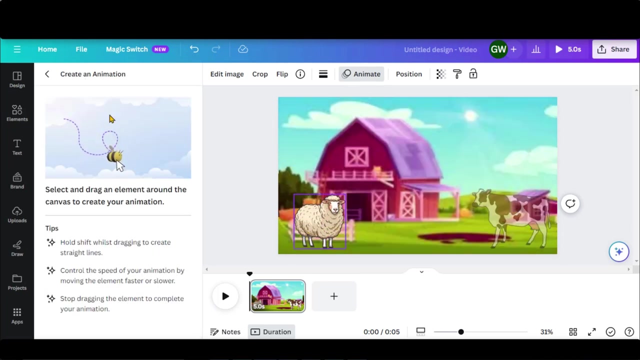 Select any of the images, Change its direction by clicking here And adjust it accordingly. Another cool feature of Canva is creating animation. Just select your image and choose the Animate option. You can choose the predefined animations. Select this, Create an animation option. 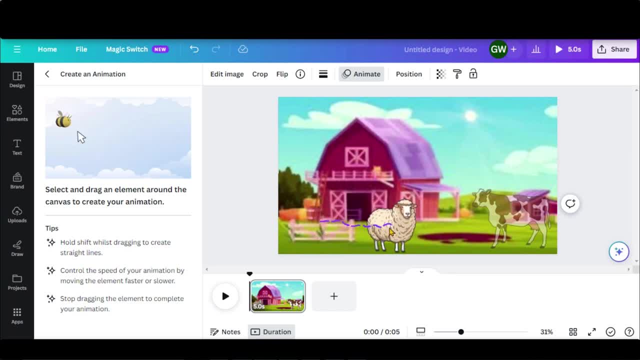 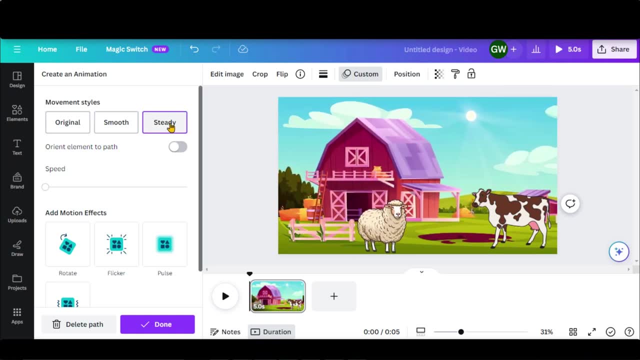 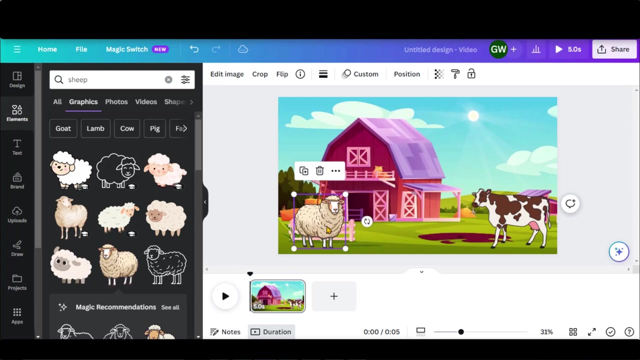 Now move this image step by step by holding the mouse key. Here you can see the animation. Choose a smooth or steady option. Similarly, select this image and create animation. Let's have a look at the final output. That looks amazing. You can also add some motion effects as well. 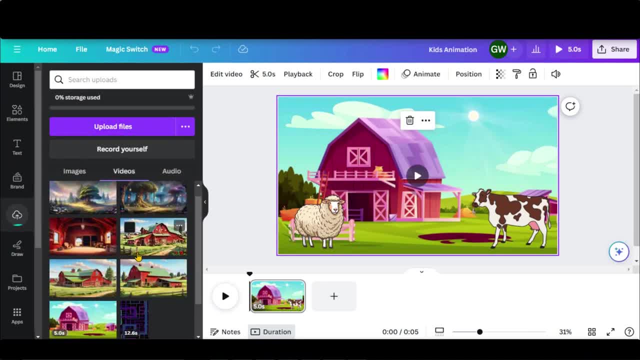 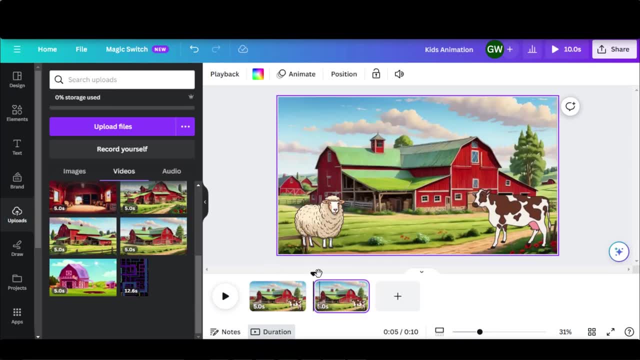 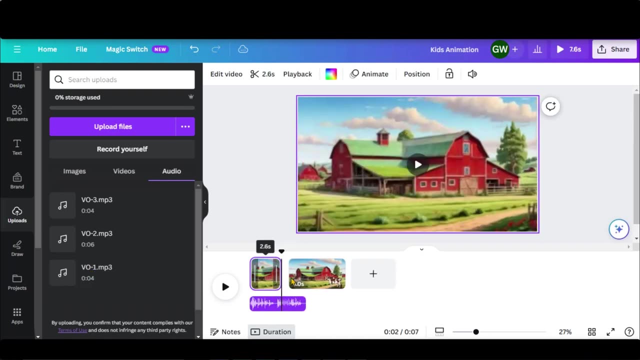 Now upload all the animation we have generated with Layapix. Replace the video with the videos of our script. Now duplicate this page. Delete the images from the first page. Upload your voiceover. Now adjust the animation and images with the voiceover. 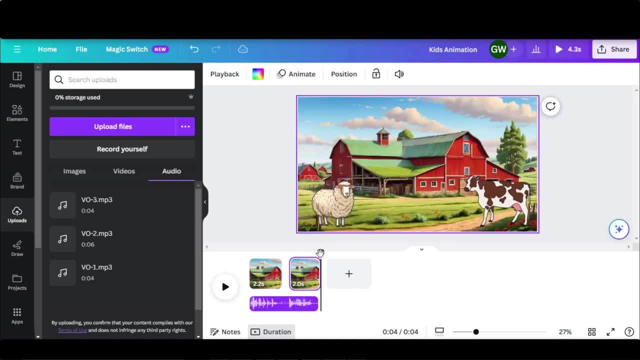 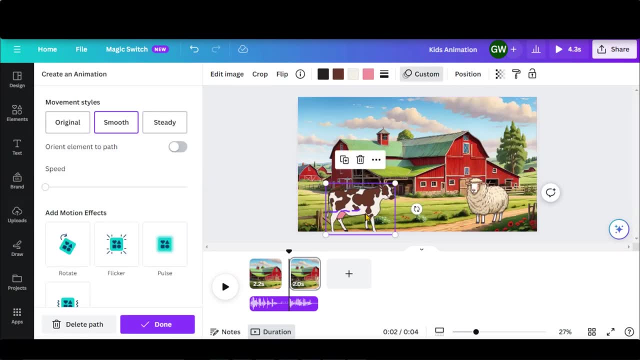 Today we'll follow two special friends: Daisy the cow and Benny the sheep. Create a duplicate page And add the second voiceover. Delete this image And adjust it accordingly. Here you can see the animation. Just click here to create it. 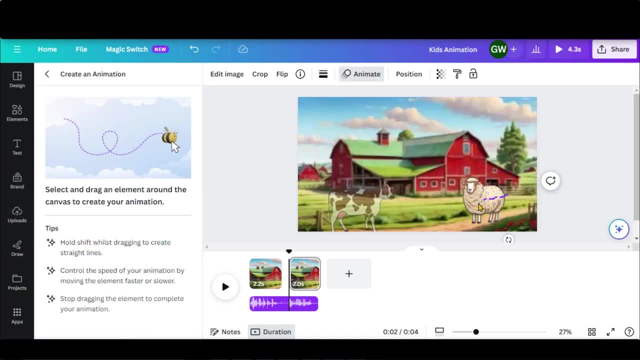 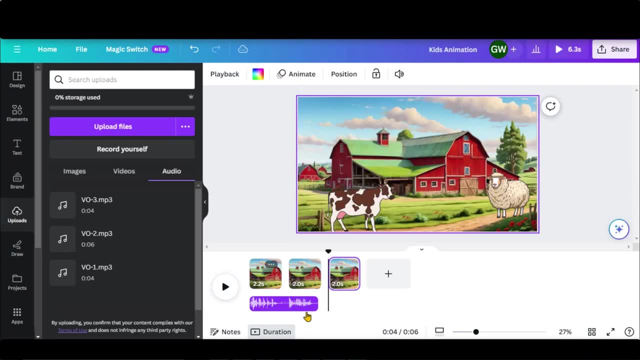 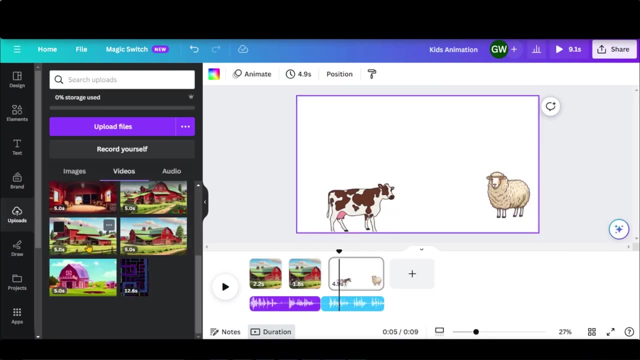 And now delete this image. Now move this image to the right side and adjust it. Delete the animation path and create it again by going to the Animate option. Today, we'll follow two special friends And add the second voiceover. Delete this background video and replace it. 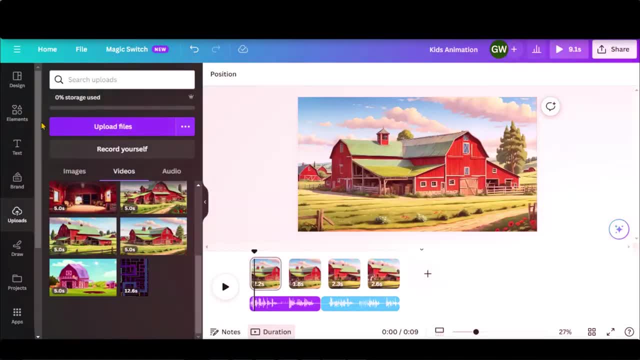 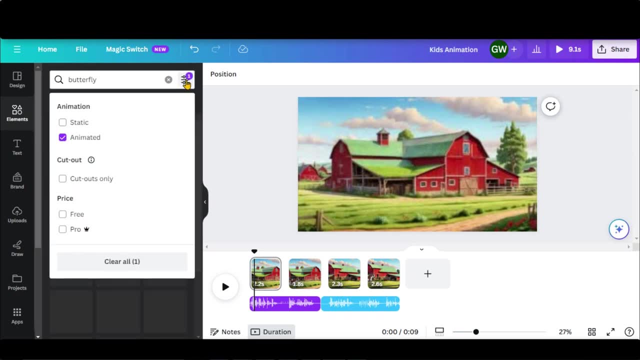 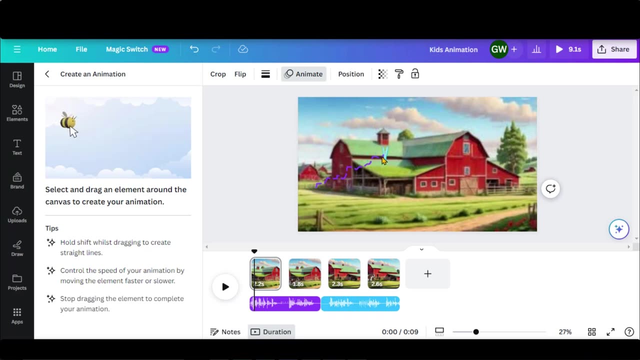 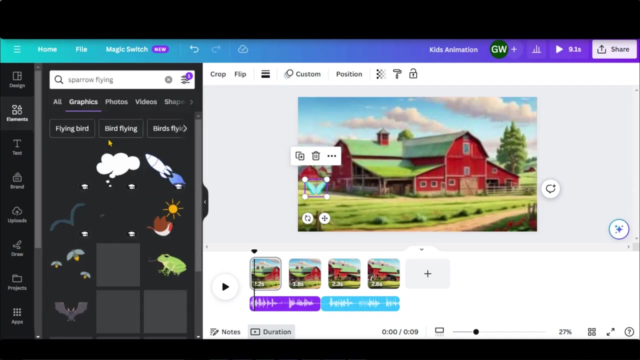 Adjust your video. You can also add some extra elements to the video, such as butterflies, birds, clouds and much more, to make it realistic. Here we have added the butterfly and sparrow. Create the animation and adjust them. Now add the background music, the voice-overs and the music.